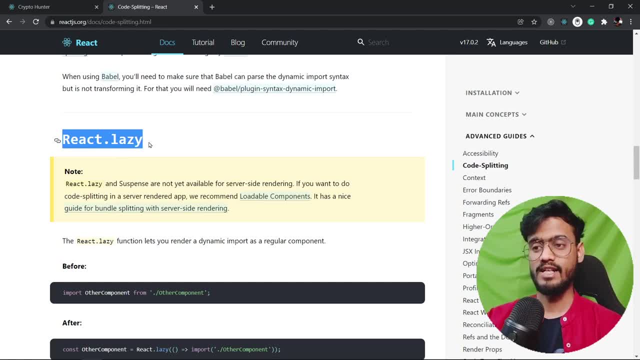 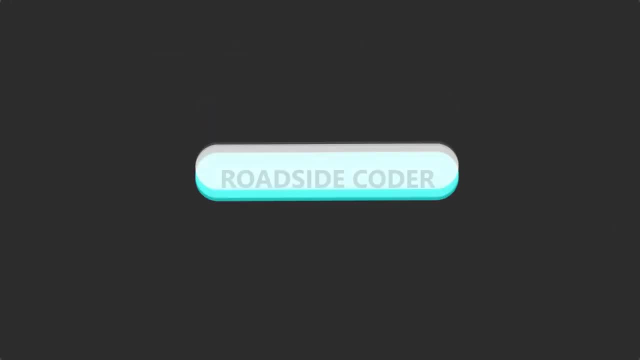 from react js. So what we're going to do is we basically have to spear in dot with react js to lazy load our app, which helps us in code splitting. So let's go on and have a look how we can implement this code splitting into our react projects. 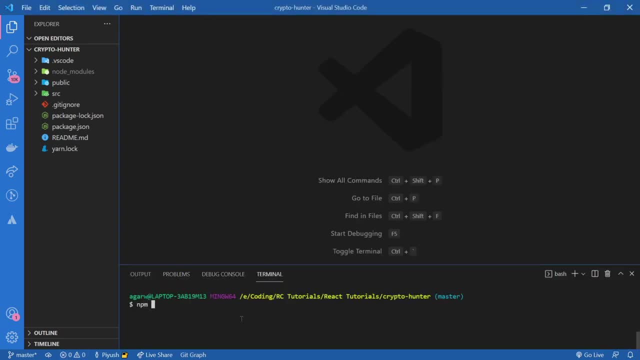 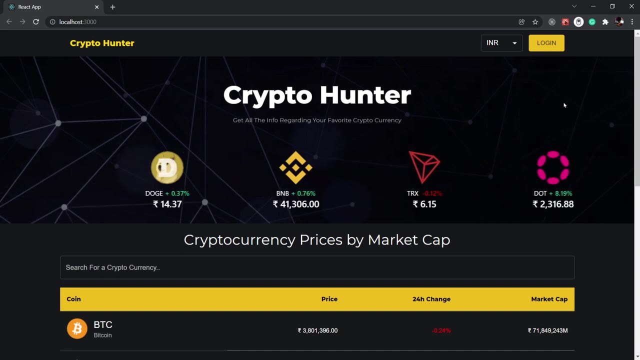 So here I've opened the project folder for our crypto hunter project. so let me go quickly to the terminal and start our app by tapping npm start. So here's our crypto hunter project. Now, if you don't know anything about this project, that's completely fine, you can still follow along. 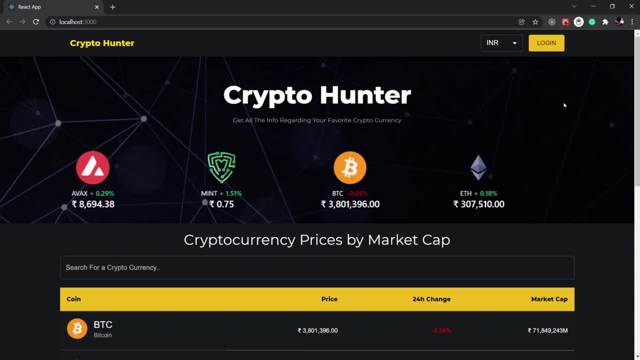 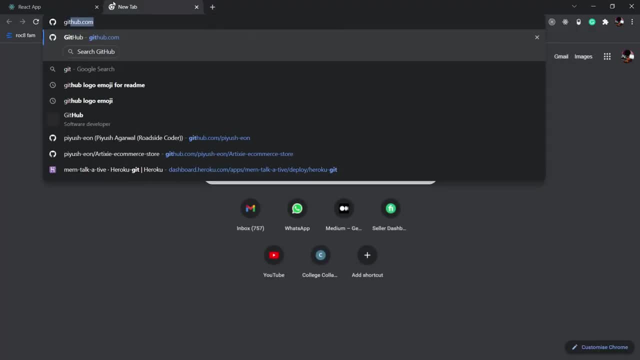 code splitting, Or if you want to go on and follow this complete project, you can check out this video link will be in the description below. But if you don't want to follow the complete project, you can go to githubcom slash, push on and here inside the repositories, If you go on and search. 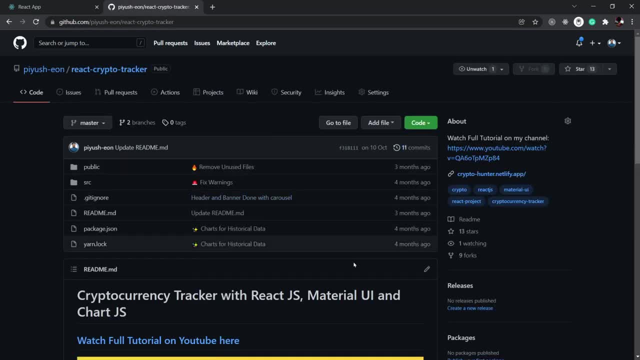 crypto. you will find the complete code to this project in this repository. Now, if you see this repo, you will see that there are multiple branches over here. you need to go to Firebase integration and just for this branch to follow along with this video, Or if you want the code. 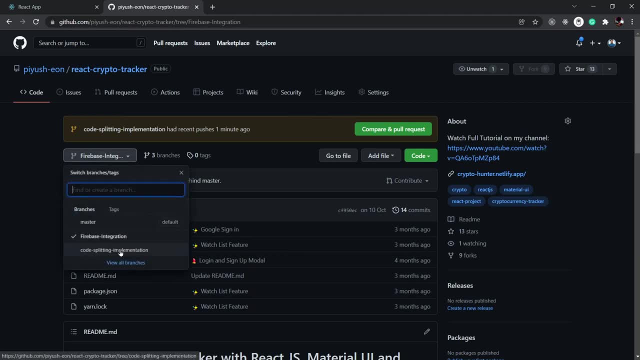 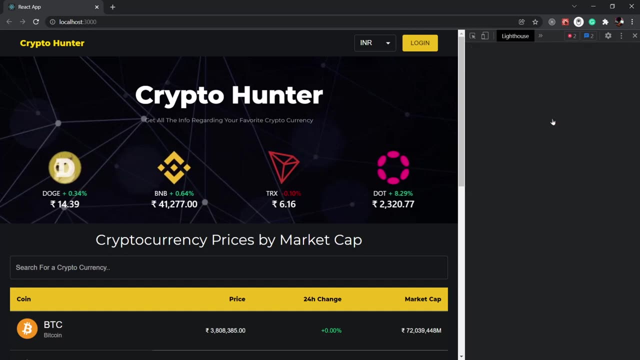 that I'm going to explain in this video. you can find that code in this code splitting implementation branch. Now, before moving forward, what I would like to do is I'm going to go to over here inside of lighthouse And I'm going to generate a report to compare the before and after result of 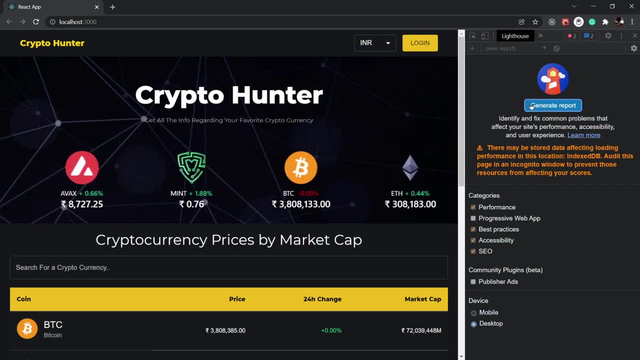 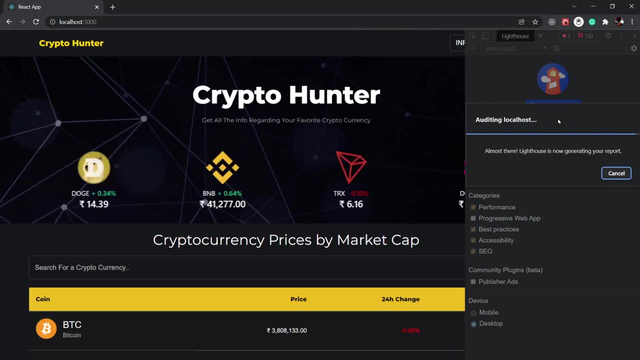 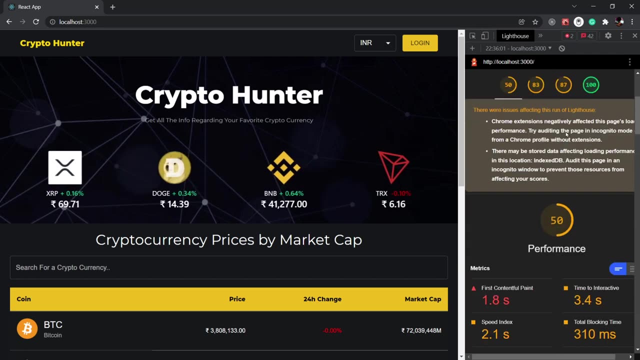 optimizing our app with code splitting. Okay, so just click on this, generate report And let's see how fast is our website right now. Okay, so these are the results that we got: performance, the 50 number. accessibility: 83.. So let's see if, after optimizing our app, does these result increase. So I'm just going to keep. 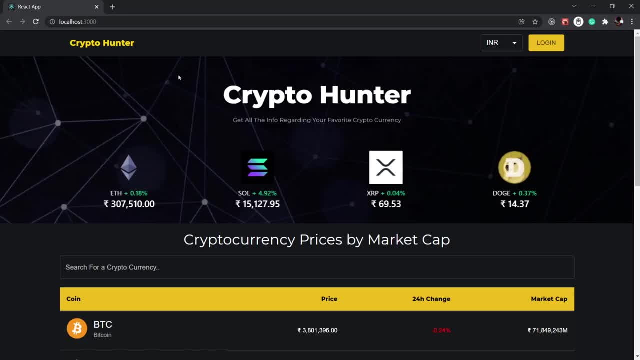 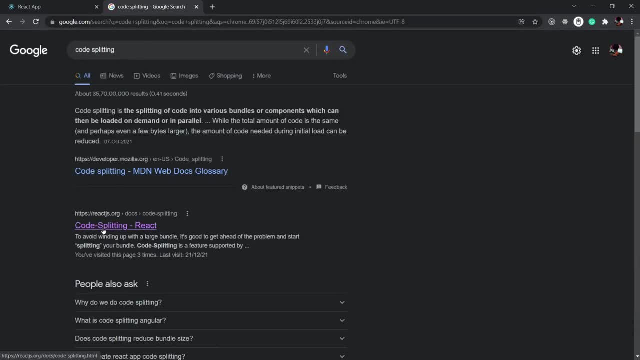 this window open like this And I'm going to open another window. So I'm going to quickly go to Google and search code splitting And you're going to see that we have this first link which will take us to the react document. 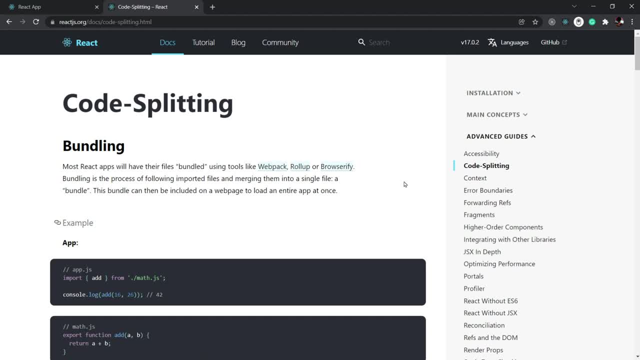 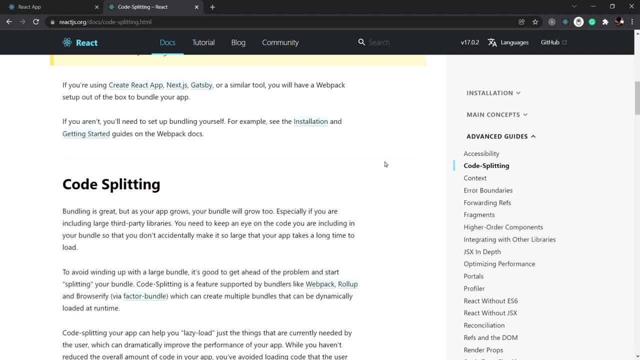 And it's explaining the same thing that I just explained you at the start of this video. So tools like webpack rollup or browser fire help bundle our react js apps and the code splitting help us to reduce the load of those js files. So if we come down over here inside of this code, 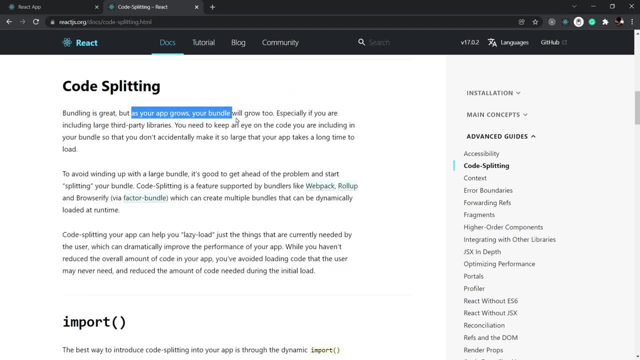 splitting, you're going to see that it says: as your app grows, your bundle will grow too. So that's why you need to split your code and lazy load your components so that your app of all forms really, really good. So then if we come down, you're gonna see we have this reactlazy. 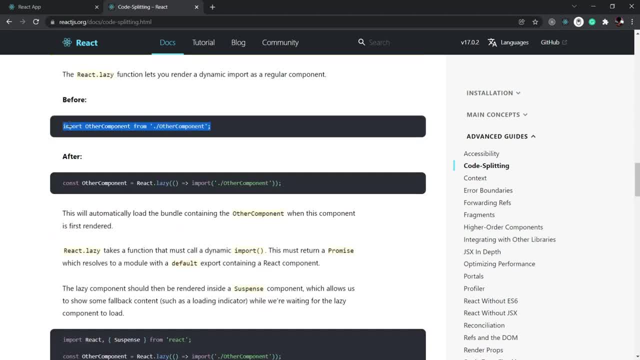 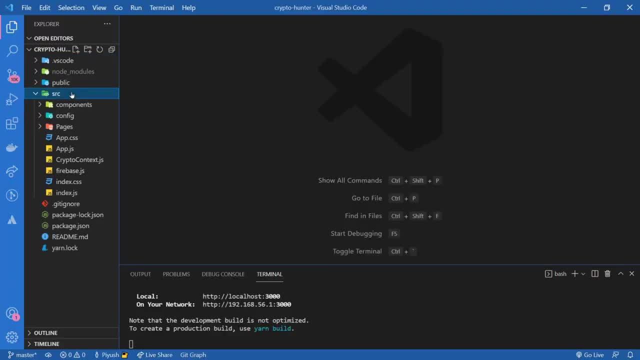 Now what is this? So we don't just import component directly, we use something called reactlazy to lazy load the components. So let me show you in the code. So if I go inside of the CRC, inside of the pages in Homepage dot js, you're gonna see that I've rendered two components over here. first, 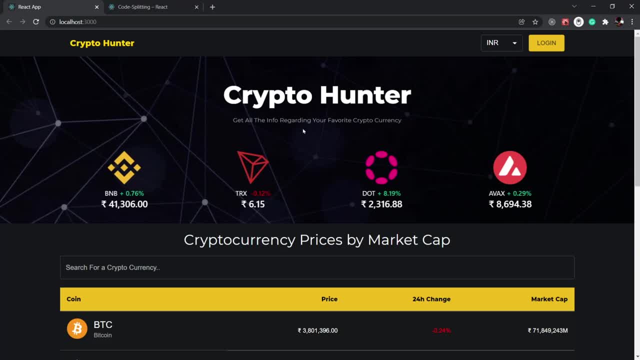 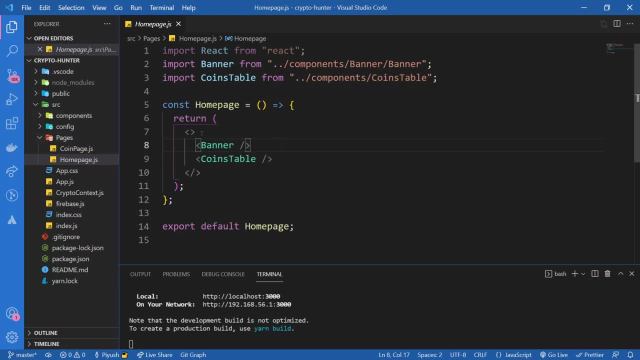 is for banner, The other is for coins table. So this is the banner and this is the coins table component. So what I'm going to do, I'm going to go on and lazy load the coins table component. So instead of this fragment, I'm just going to add a tab over here And I'm going to say const. 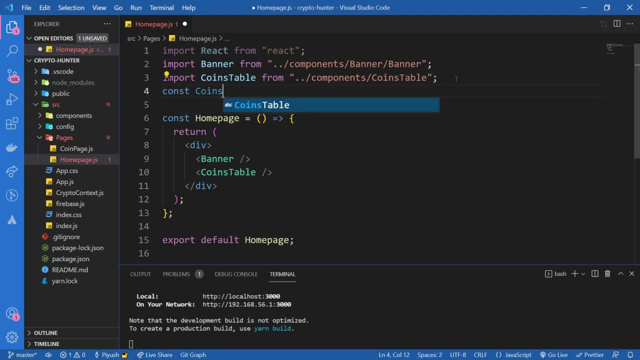 coins table equals. and I'll say react, dot, lazy, And inside of this we're going to take this path. And we're going to say import, And inside of it I'm going to provide that path. So this is how we lazy load a component. So let me remove this line now And let's check it out. 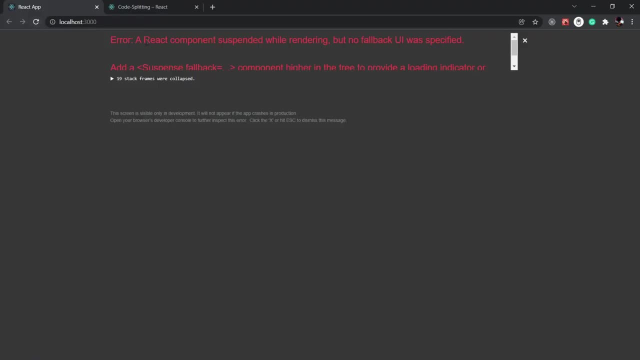 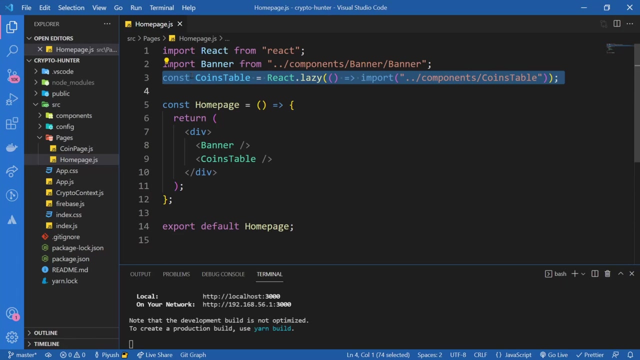 Okay, so we have another error: a react component suspended while rendering, but no fallback UI was specified. So what does this mean? So this means that this component was lazy loaded. Okay, that's fine, But while this was lazy loading, it should have something. 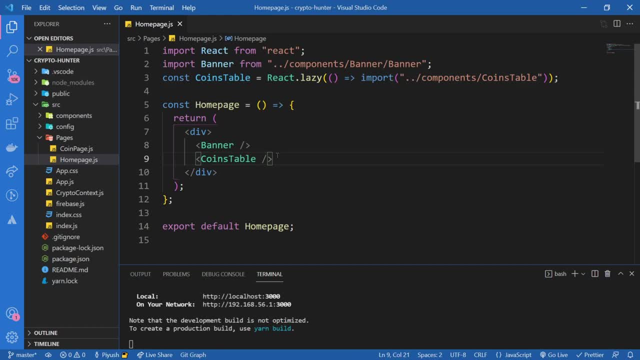 to display. right, It shouldn't be just empty. it should display something like loading or, you know, also like a spinner or something like that. So we need to use something called something Suspense now. So let's go to the documentation and see what suspense is. So okay, we did just. 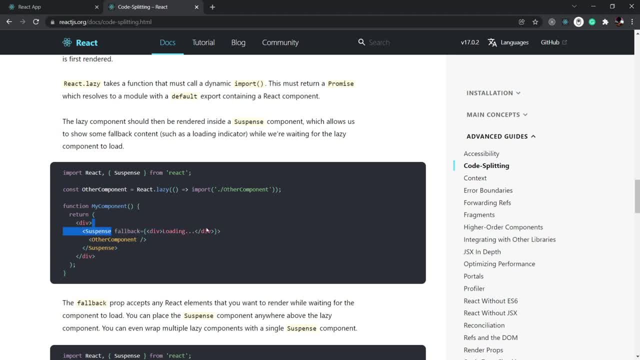 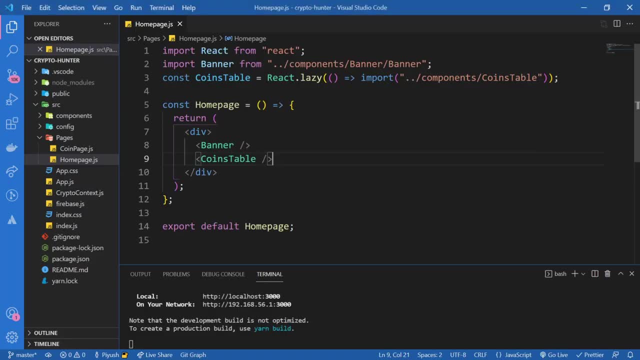 like this, But we need to wrap it with something called this suspense, which comes from react. So, okay, fine, Let's copy this line up and try this out. I'm gonna wrap this and put it inside of over here And let's import suspense from react. Yep, just like that, Save this. 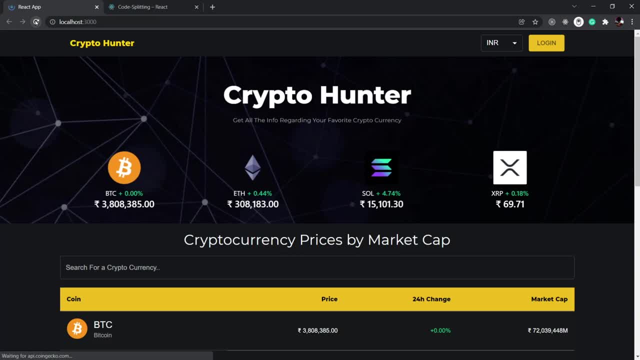 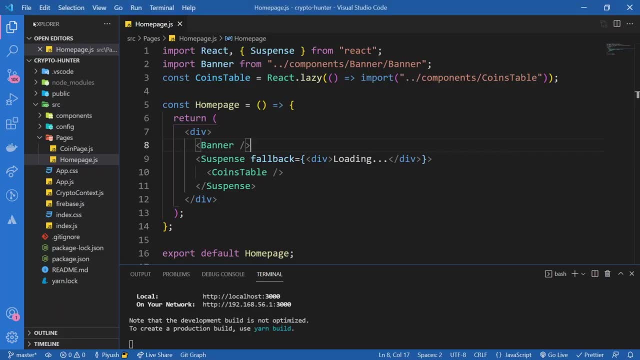 And let's see if our app works fine. Yep, it does. Let's reload. You're going to see that there is a loading over here for a split second. I don't know if you can see that or not. Where is that coming? 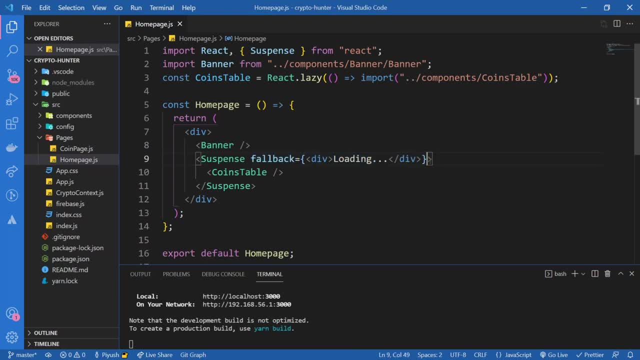 from It's coming from over here. inside of this fallback you can give another component for loading. you can give any sort of custom component or stuff like that. I've just given a div with the text of loading. So this is our fallback UI. this UI will be displayed while this component is being 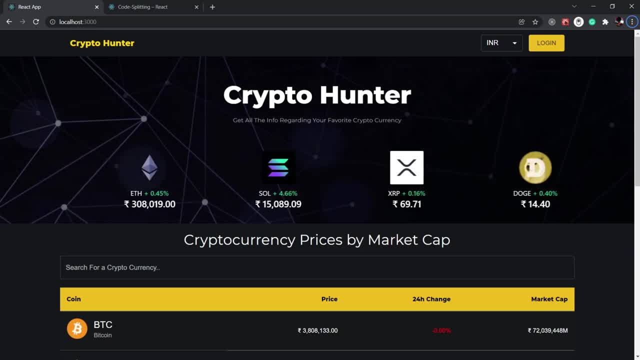 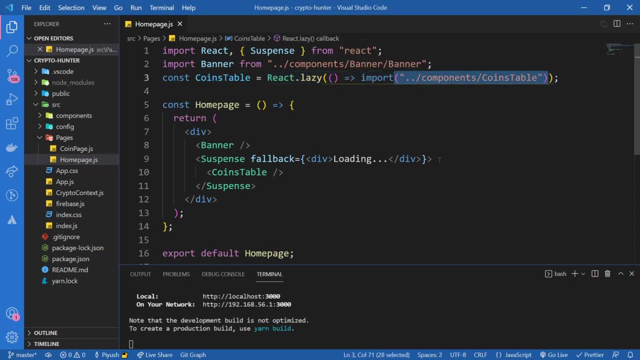 lazy loaded. Okay, so you've understood what the basic lazy loading is. we just add this reactlazy and import this component inside of it, And then we provide it a fallback UI by using suspense. But what if, while lazy loading, our component fails to load for some reason? then we need to handle. 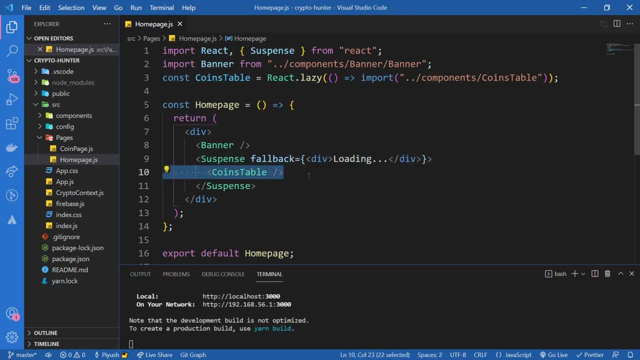 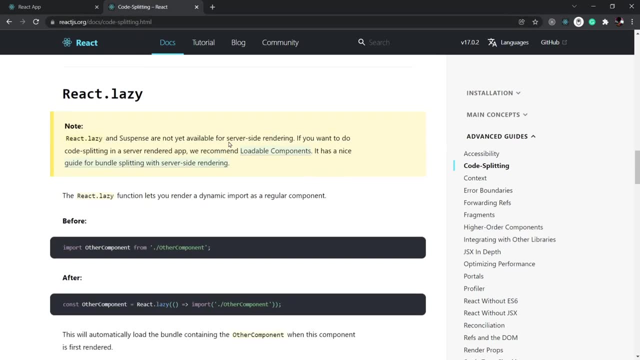 that error right. We need to display some sort of error, So that's why we use something called error boundaries. So let's see what error boundary is all about. So if we go back to our documentation, you're going to see that next is 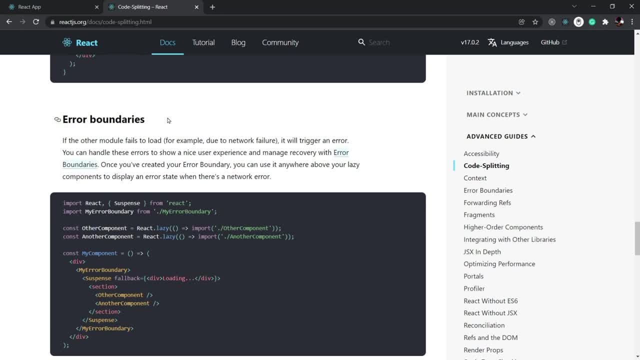 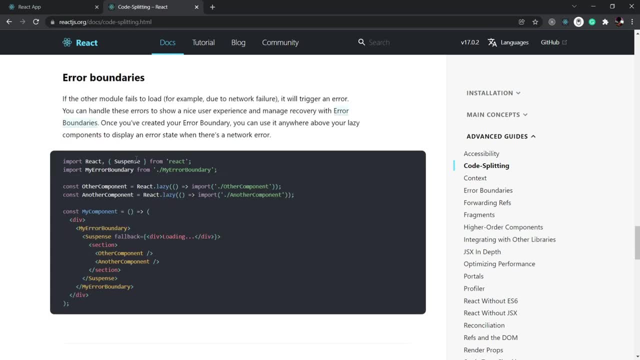 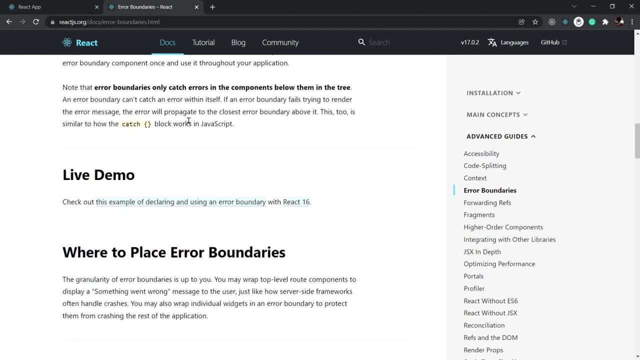 error boundaries. So to implement error boundaries, we just create a component for our error boundary and we just wrap it on the lazy loaded component. So let's see their example of error boundary. So I'm going to go and click on this link And instead of here we're gonna see that. 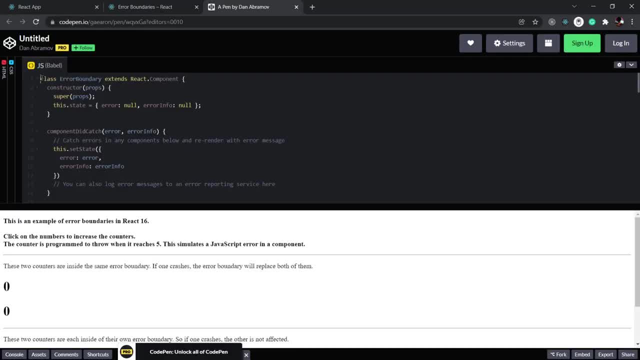 live demo. Okay, let's see the live demo. So I can see that they've given us the error boundary example with the class based component. So if you want to go on and understand the class based component, you can go on and understand. 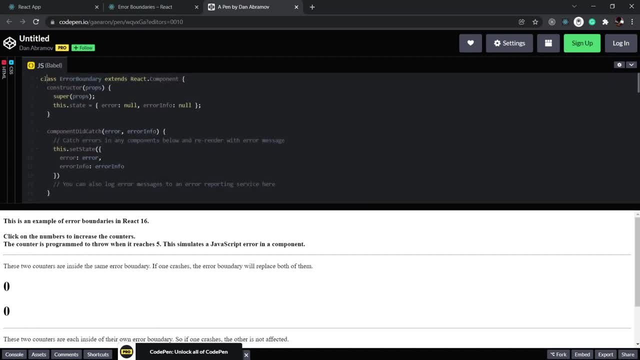 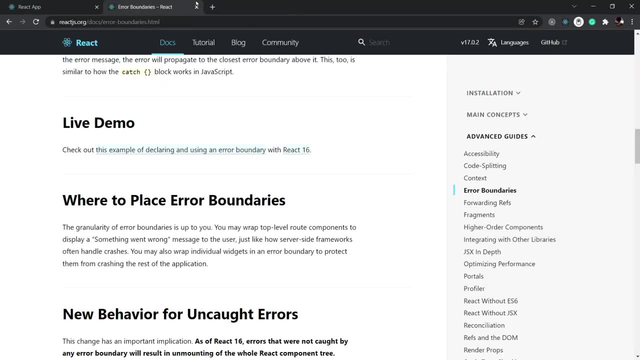 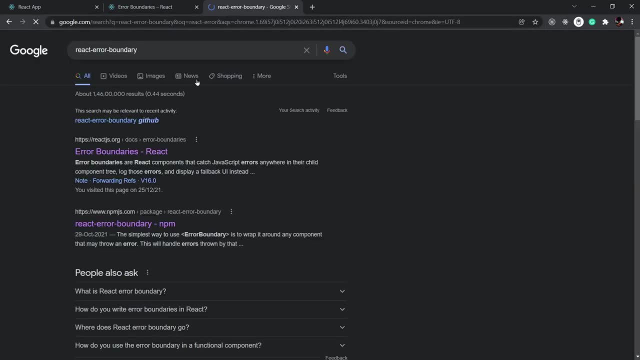 This error boundary that they have provided, but I'm going to explain you how to create your own error boundaries in a much more easier way than this. So I'm just going to close this up And I'm going to go and search react error boundary. So this is an NPM package. 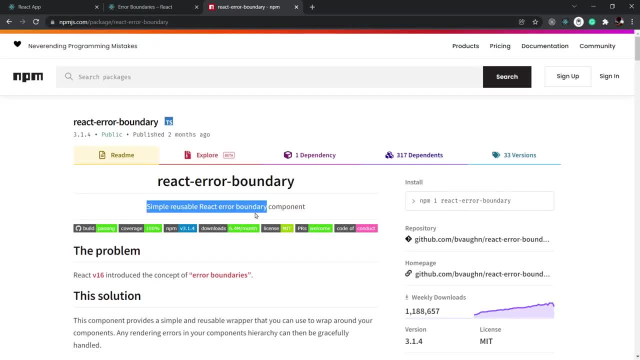 So let's open this up. Here we go. So it's a simple, reusable error boundary component- Awesome. So we don't want to create our own error boundaries and, you know, create a lot of hassle. But in this case, this is much more simpler than that, So I'm going to copy this and install. 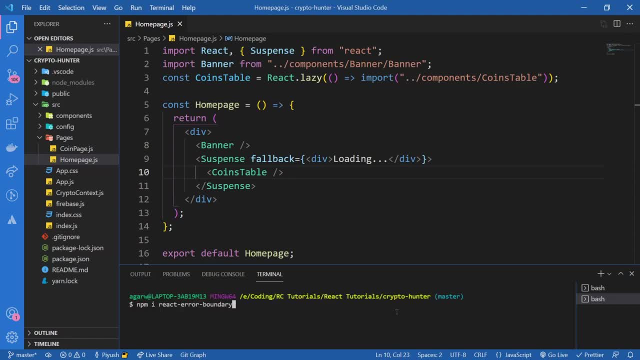 it in our project, So I'm going to open another terminal and paste it. Alright, reactor: boundary has installed. let me close this terminal up And I'm going to create an error boundary for this component. So I'm going to go inside of the components folder and create a new. 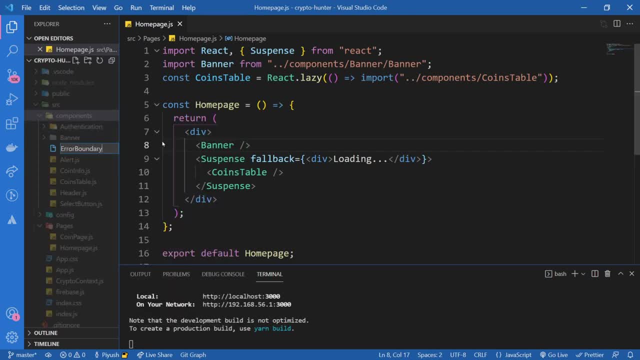 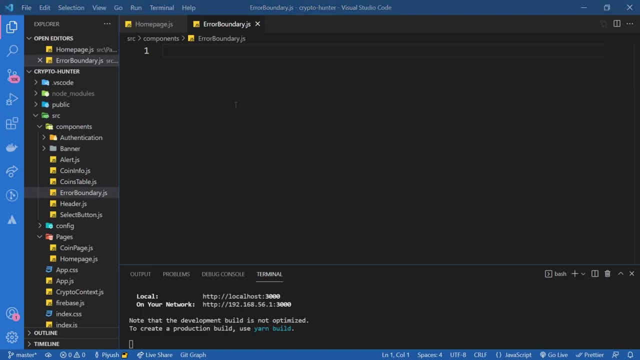 file called error boundary, dot j s, And inside of this I'm going to create my own error boundary. So let's go to the documentation for reactor boundary. So let's go to the documentation For reactor boundary and see how they have told us. So. okay, this creates a function. 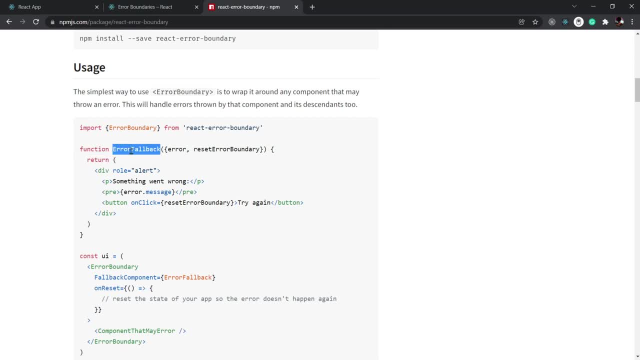 called error fallback And obviously you can give any name to this function And it takes an error and a function to reset that error. Okay, And so this: they have created this simple component to display this error. Okay, fine, Let's, let me just copy it up. 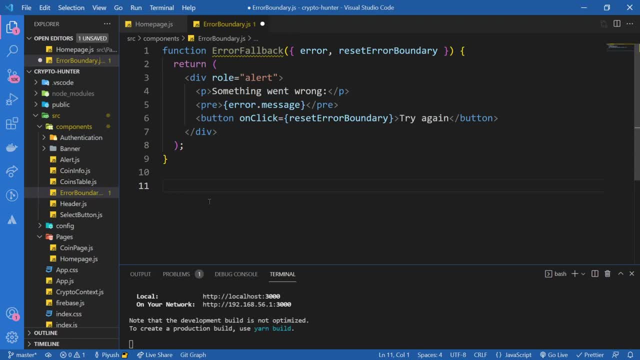 Because this is self explanatory and I'm going to export it. So export default error fallback- Awesome. So again they have given this. something went wrong and just display the error message and a button to reset the error boundary, which I'm going to explain. 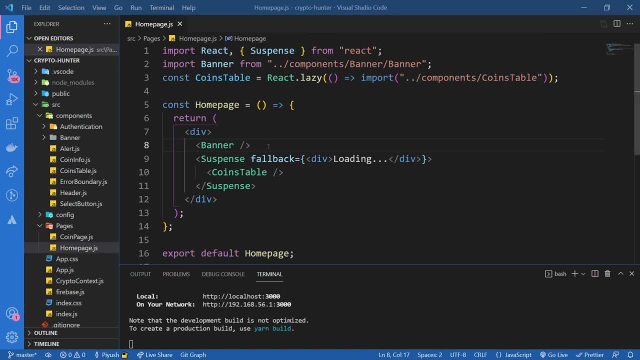 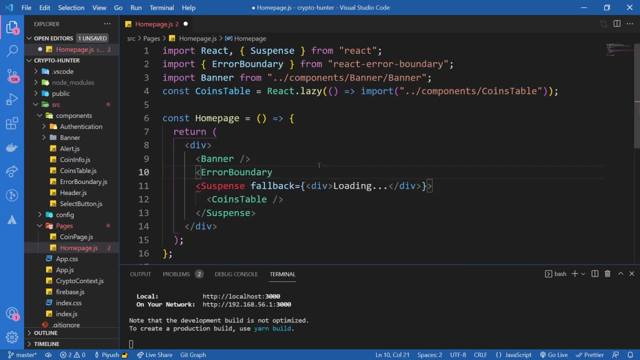 how we're going to provide it that function. And now I'm going to come over here and wrap this in something called error Oops, error boundary, which obviously comes from reactor boundary. So just like this: Cool. Now this takes a bunch of props, So let's go ahead. 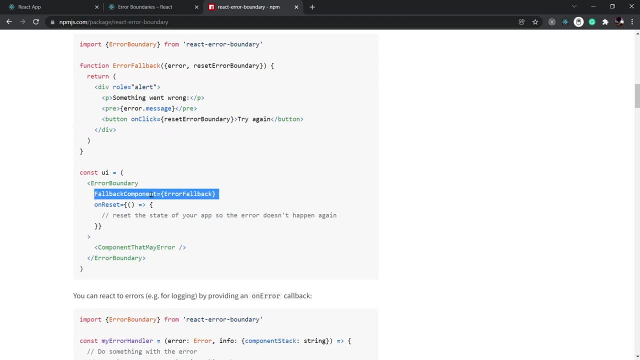 Let's see. It takes a fallback component, which means whenever the error occurs, it's going to go and display this component, which is this component that we just created over here. this one And the other thing that it's going to take is on reset, which will contain: 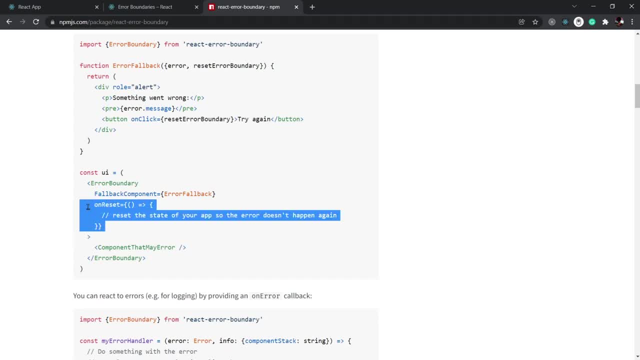 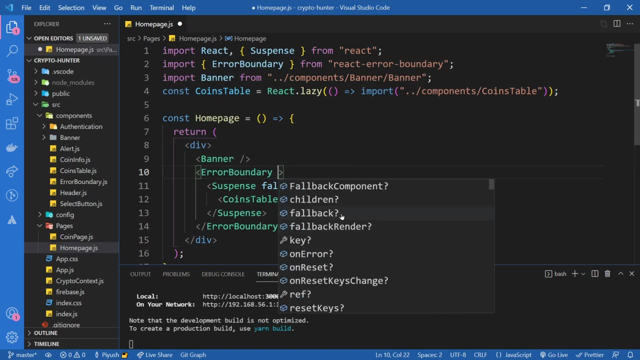 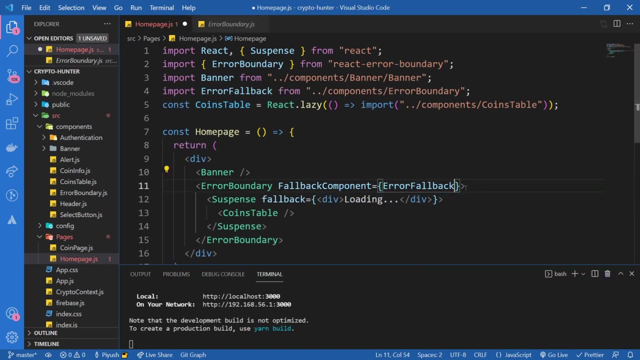 the logic for resetting the error, And I'm going to come to that later, don't worry. So, okay, we close this and I'm going to provide it Fallback component, which is going to be error Fallback. Yup, there we go. We have imported this, And the other thing that it takes is: 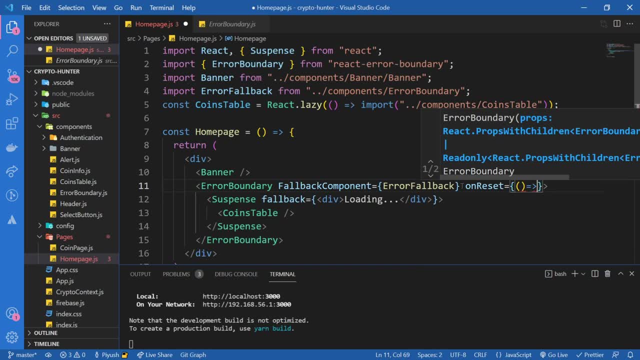 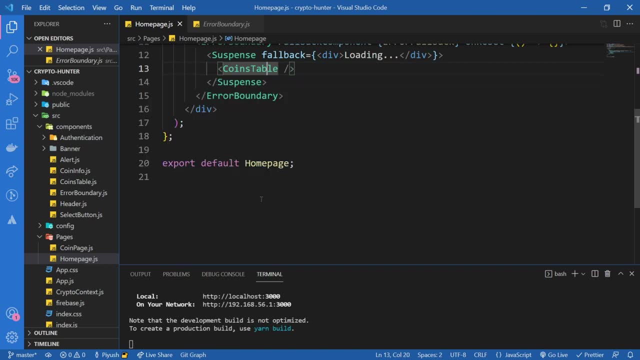 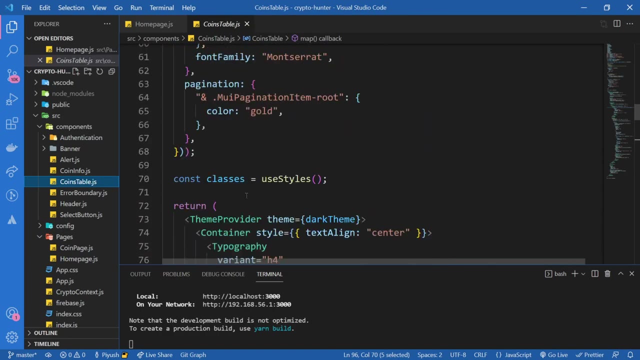 on reset, which I'm just going to keep empty like this. Cool, Let's simulate an error. probably Let's go inside of this coins table component. So, over here, And what I'm going to do is just above this return statement, I'm going to write: 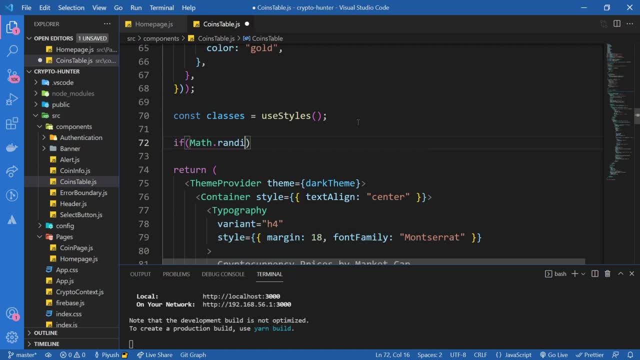 if math dot random, which generates a random number between zero and one. So I'm going to say, if it's more than 0.5, then throw the error, because obviously it's not going to be more than 0.5 every time. 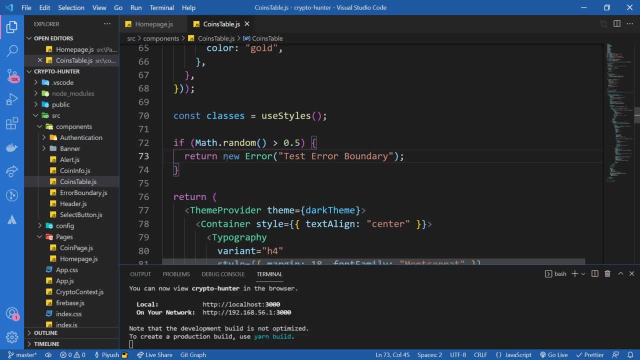 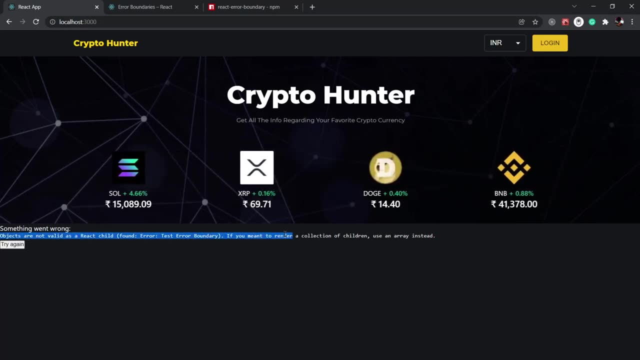 So sometimes it's going to throw error and sometimes it won't, So let's save this and check it out. So, yep, you see that it threw this error. objects are not valid as react child If you're meant to render a collection. blah, blah, blah. 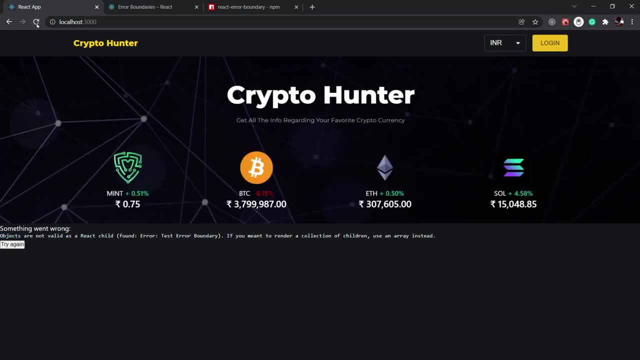 And if I refresh it we'll see a lot of error, And so if we refresh it, So we're just basically simulating an error over here. Obviously, this is not how the real app works, But we're just simulating an error over here to show you what happens if a component, while loading, throws an error. 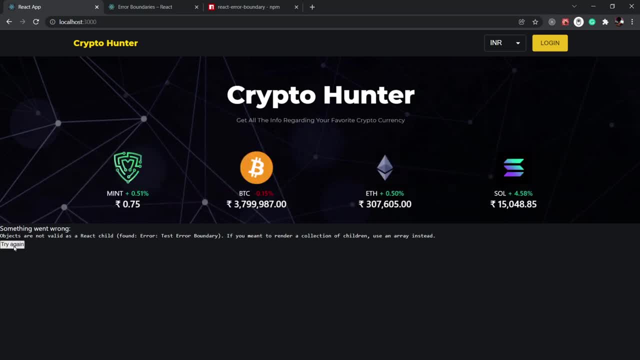 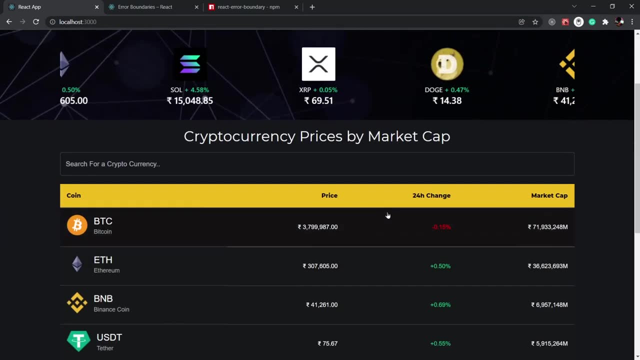 Now, if I click on this try again, it's going to generate a random number every time. So, yep, so this time it generated the number below the 0.5.. So it displayed as this component. So this is how we handle the errors in lazy loading by using error boundaries. So let's. 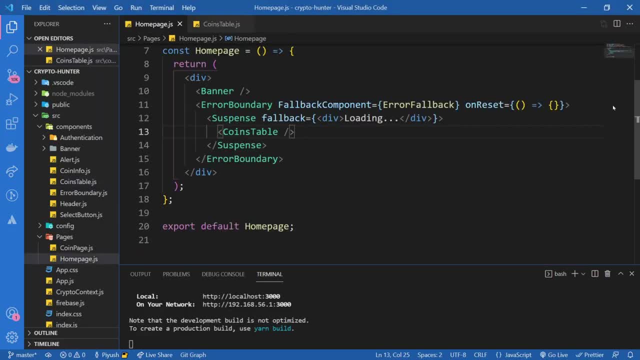 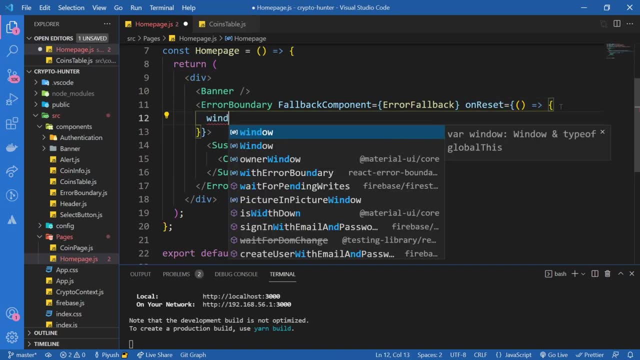 let me go over here And inside of this, on reset function, you can write any logic for resetting your error. For example, in this case I'm just going to write window dot. location, dot, reload- I'm just going to reload the app. Or let's say, if there's a particular state that's giving us. 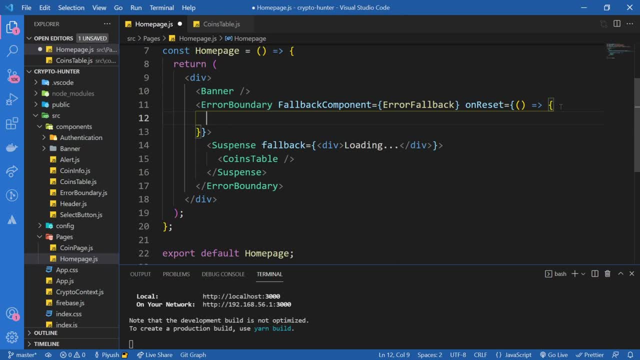 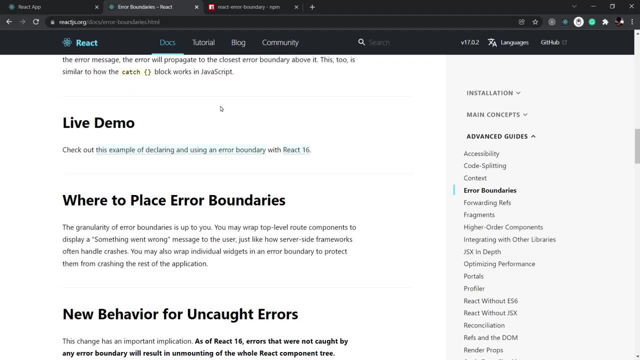 this error, we can reset that state. So I think you got my point, what I'm trying to say. So this is what error boundaries, and obviously I would highly recommend you to go and read more about this in the official react documentation. This will clear your doubts much, much more. Now let's. 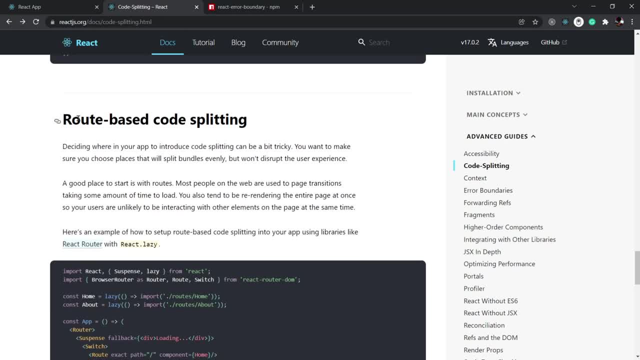 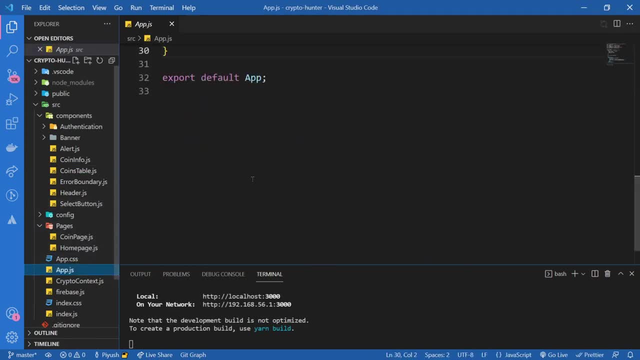 move further and see we have route based code splitting. So what is route based code splitting? So, inside of our app, if we go inside the app dot j s, which is right here, we have two pages, homepage and the coin page, And when the app loads, the whole j s chunk loads both of these. 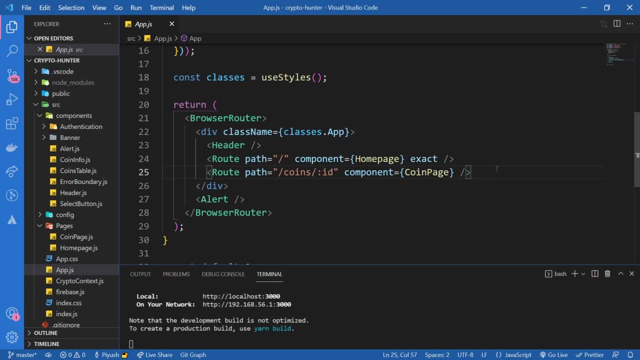 pages, so that our app is very fast And whenever our app starts it loads the whole chunk of j s containing both of these pages. But what if we manage to only call the j s chunk whenever we go to that particular page? right, So that is what we want to do. So that's why we're 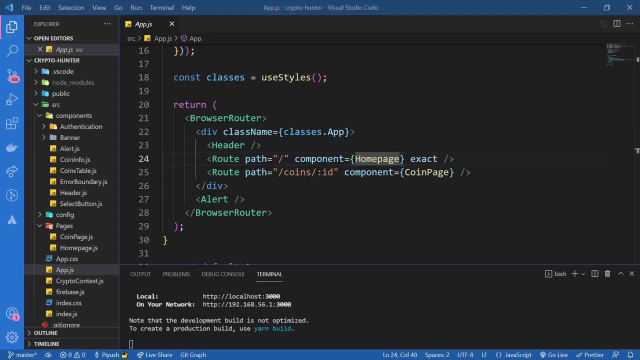 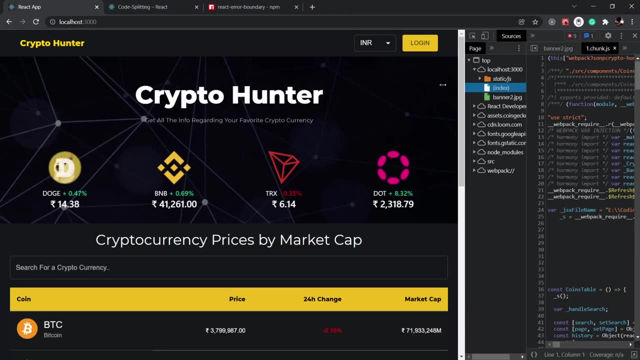 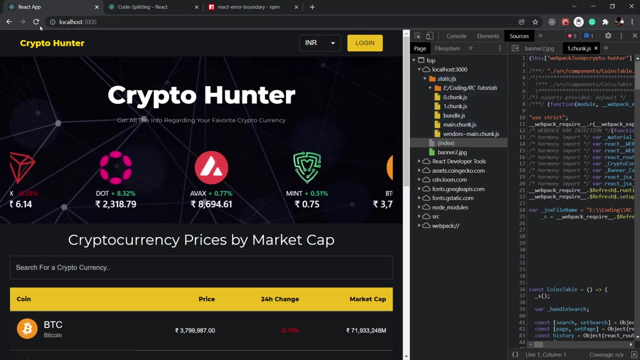 going to use route based code splitting. So if we go inside of our app, and I'm going to go to inspect inside of sources, you're going to see we have this j s file right, Just j s folder. Inside of this we have these bunch of chunks. So if 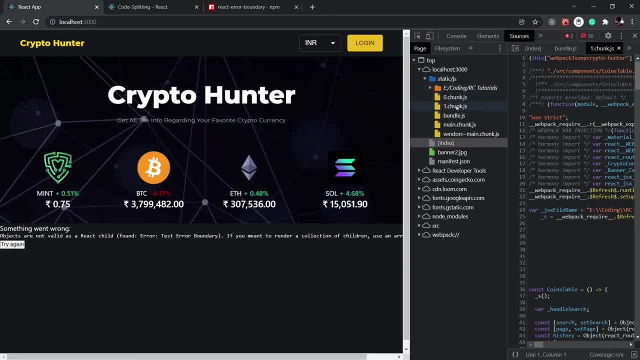 I reload our page. you're going to see when our app loads. it loads all of these chunks of JavaScript, these huge chunks of JavaScript. But now watch this. what's going to happen? So if I go over here and lazy load both of these pages, 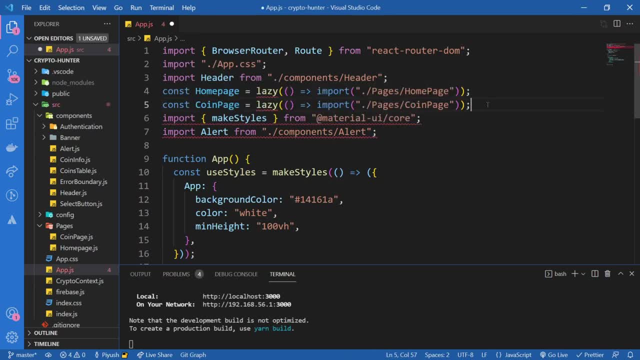 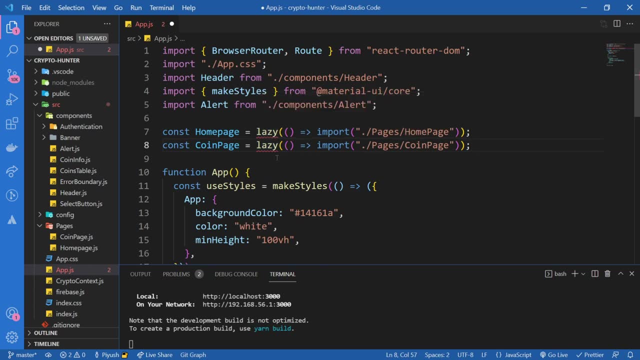 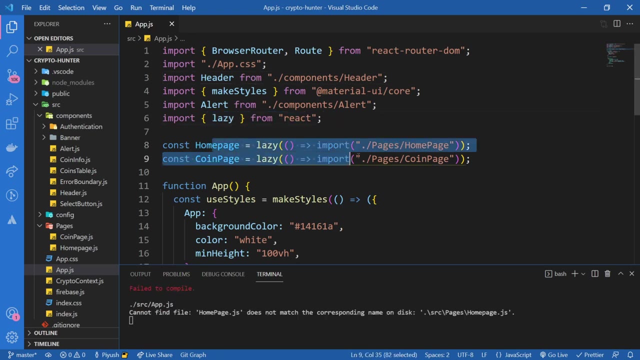 So let me quickly add the react dot lazy to this, which is going to be just like this, And notice one thing: this has to go below all of the imports just over here. Okay, let me load lazy as well. Okay, cool, It has loaded, I believe. Yep, just like that. So this has been lazy, loaded, but we forgot. 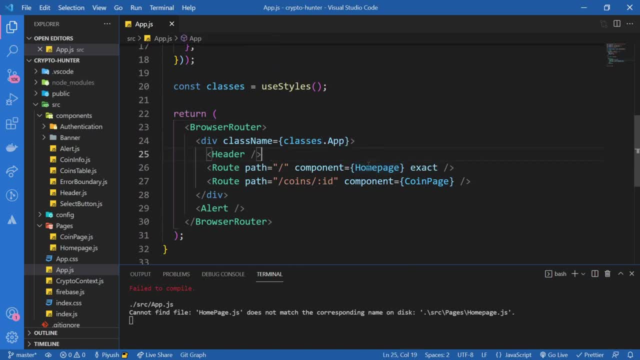 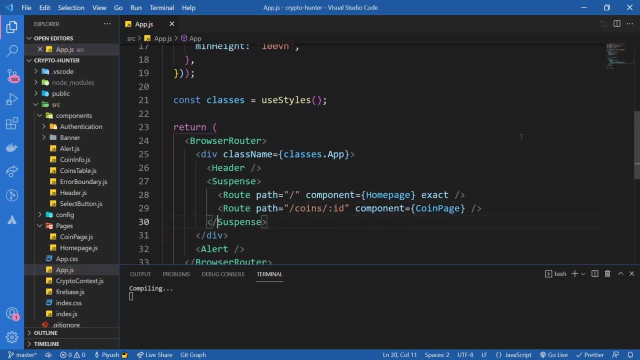 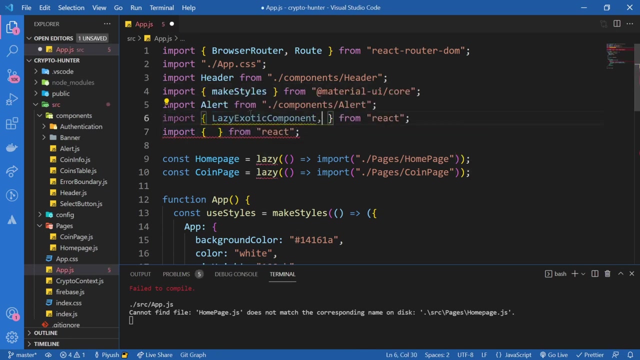 to give it the suspense fallback. So we need to wrap this with suspense as well, And don't forget to import it from react, just like this. Why has it imported twice like that? I'm gonna do this- Cool Now, this needs some fallback. So I'm going to do this- Cool Now, this needs some fallback. So 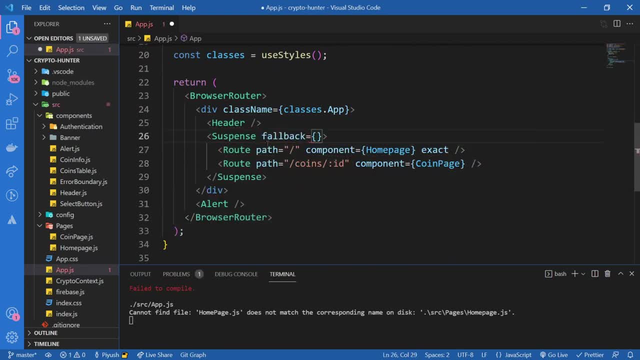 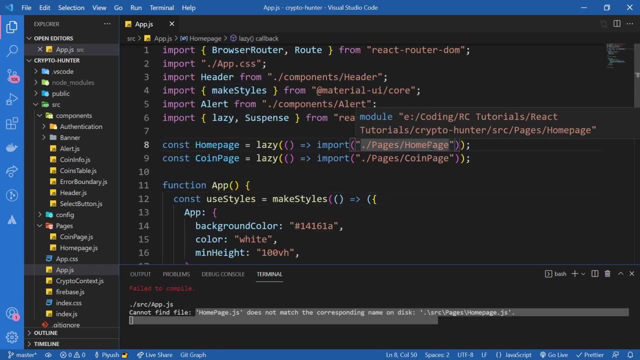 I'm just gonna give the normal div loading, So div and loading, Cool. So this should work. Okay, what's wrong? cannot find the file. Okay, so this is home page Now I think it's fine, So awesome, Let's go on and test this out. 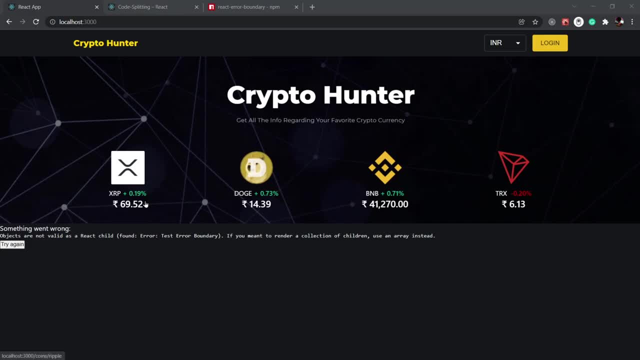 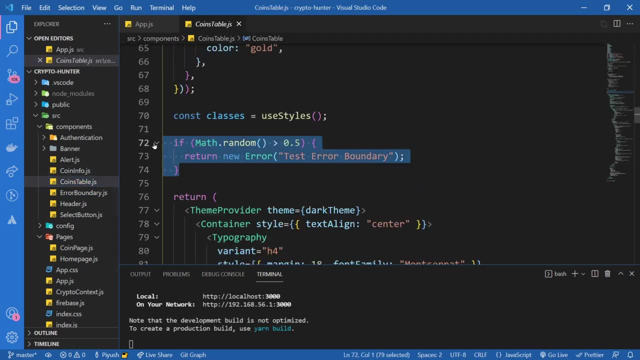 So if we go and check? so first of all, let me remove this error boundary from over here. So inside of this console table, I'm going to comment it out. we don't want to throw any error now. Okay, now if we go back to our app.